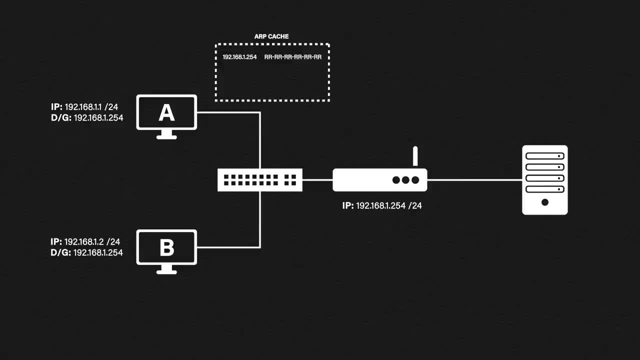 the default gateway, which, in our case, is the router. From here, the router handles the rest. Now, if this looks unfamiliar to you, I have a few tips to help you understand this. First, you can have a video explaining this process in a bit more detail, so feel free to go and check that out. 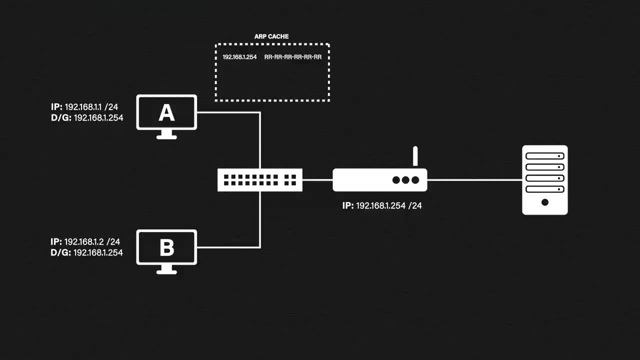 So that is how ARP is supposed to work. However, there are some flaws to this process. Let's say, host B isn't Billy Bob from down the hall. he's actually an evil hacker trying to steal our information. The hacker can send, specifically: 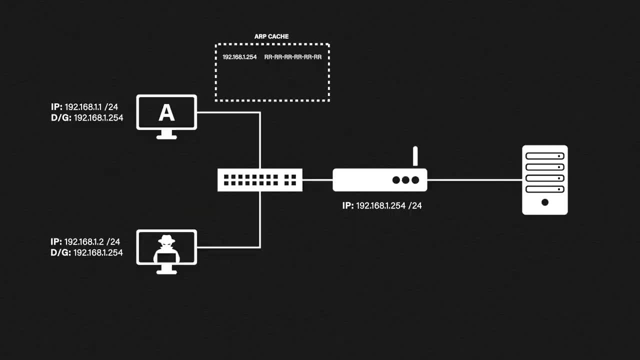 crafted ARP messages to our host, pretending to be the default gateway. The idea is to poison host A. So host A went on the app and changed host A's ARP cache and tricked it into listing the hacker's address as the default gateway. So in this case, host A replaces the MAC address for the. 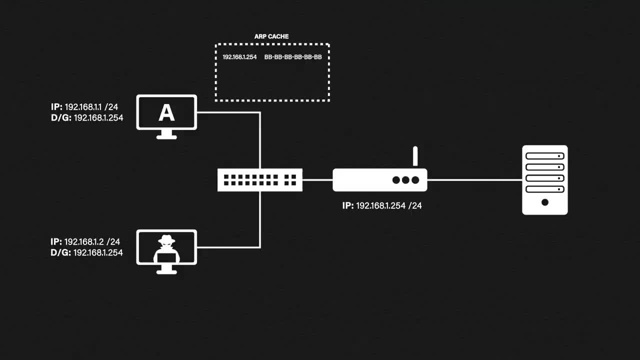 default gateway with the MAC address of our evil hacker. Now, if host A again wants to send some data to the web server, he's going to look up the MAC address in his ARP cache. The data will be sent to the switch just like before, But this time. our router. It's sent to the evil hacker instead. The hacker can now do all the snooping he wants on the data before sending it to the real default gateway. This attack is known as a man-in-the-middle attack. It's where the 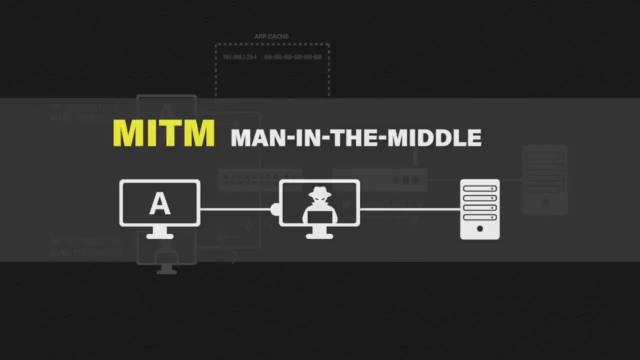 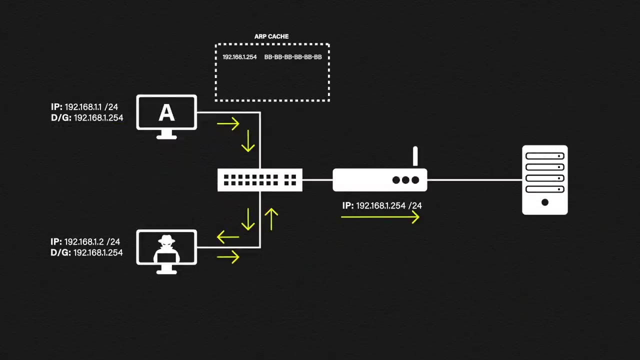 attacker places himself in between or in the middle of the victim and whichever system is trying to access, If successful, the hacker can inspect everything that is happening, while the victim is none the wiser. So that was the theory. Now let's see this in action. 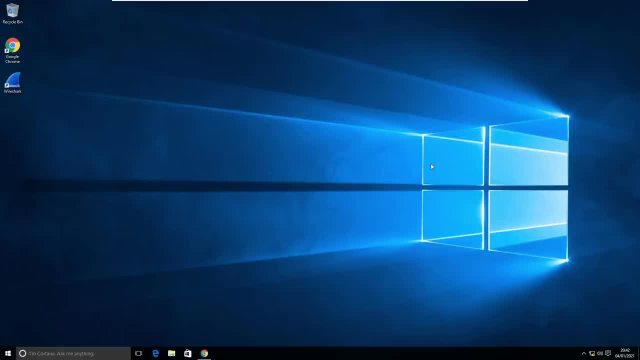 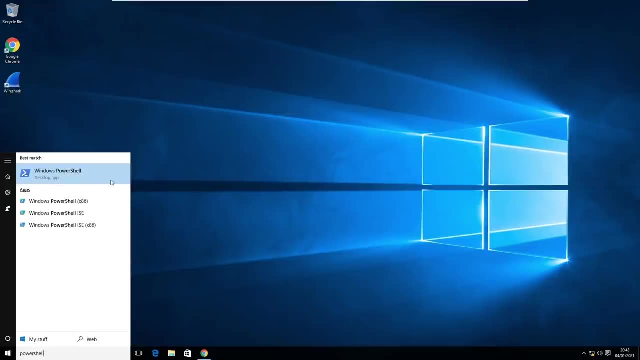 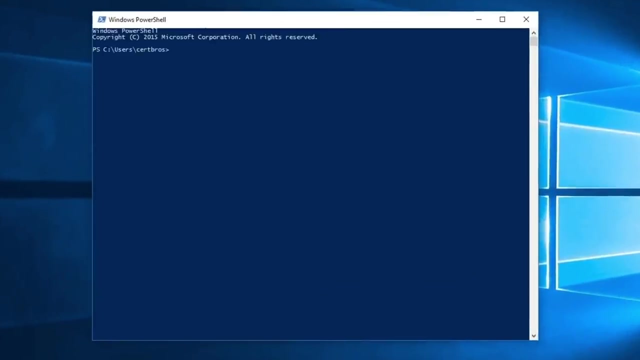 Here is our victim's computer. Before we do anything, let's just check a few things. If I go to start, then type PowerShell. move this into the center so we can all see. First let's check the IP address and the default gateway. To do this we'll type ipconfig. Here we can see the IP address of this. 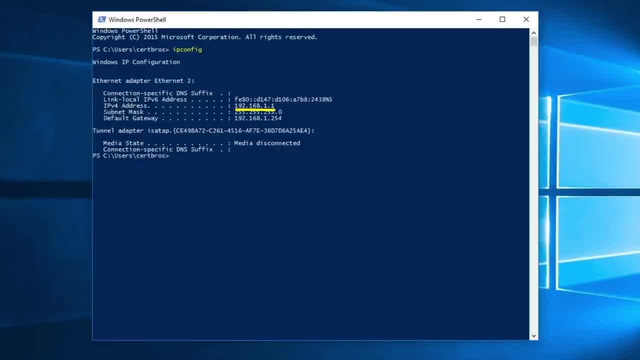 machine, which is 192.168.1.1, and our default gateway is 192.168.1.254. Next, I'm going to check the ARP cache by typing arp-a. Here we can see the default gateway's IP address and the associated MAC address. So everything. 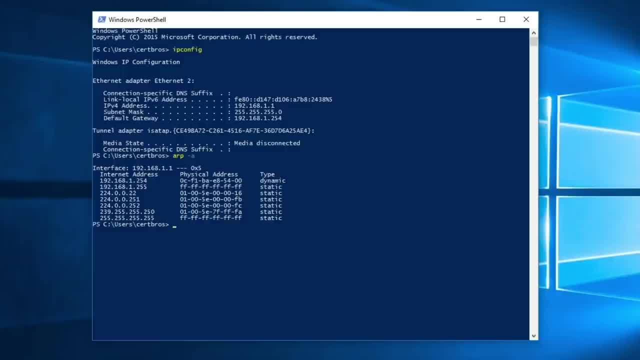 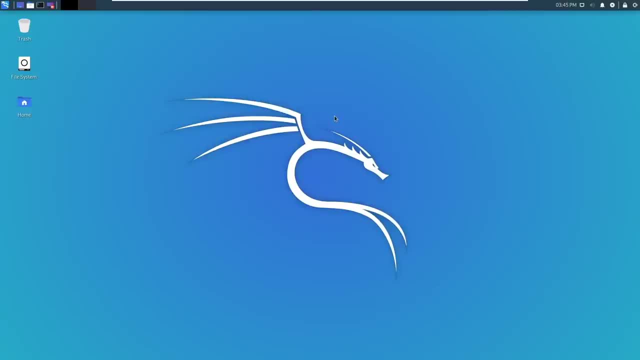 is working as it should. Let's now introduce our hackers machine. This is Kali Linux. Kali is a Linux distribution used for penetration testing or ethical hacking. Don't worry, if you're not familiar with Linux, you can still follow along to get the idea. The first thing I'm going to do is open the terminal and 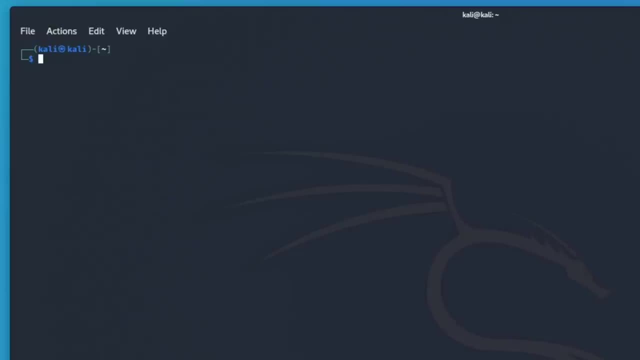 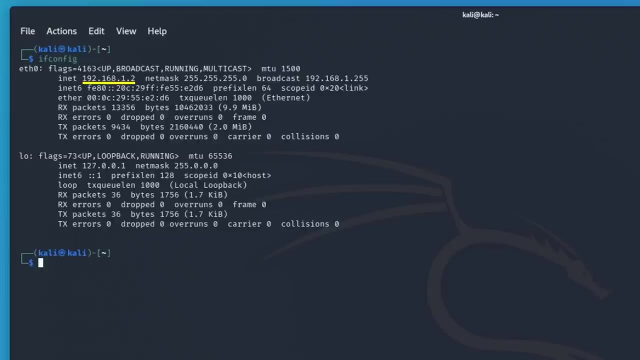 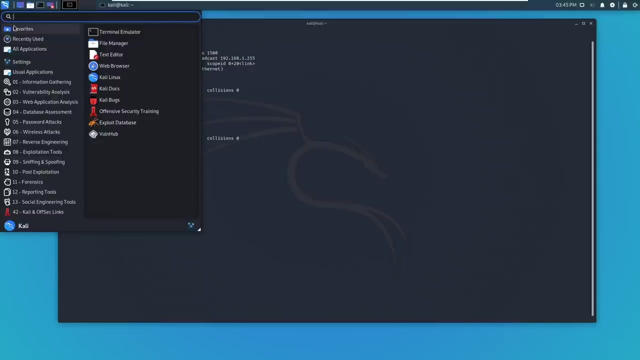 just like with our victim, I'm going to check the IP address by typing ifconfig. As we can see, this machine has an IP address of 192.168.1.2.. We can also see the MAC address here. Take a mental note of this. Remember it ends in d6.. So now I'm going to open the menu go. 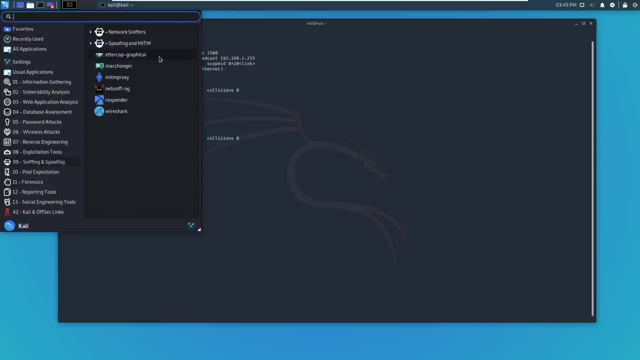 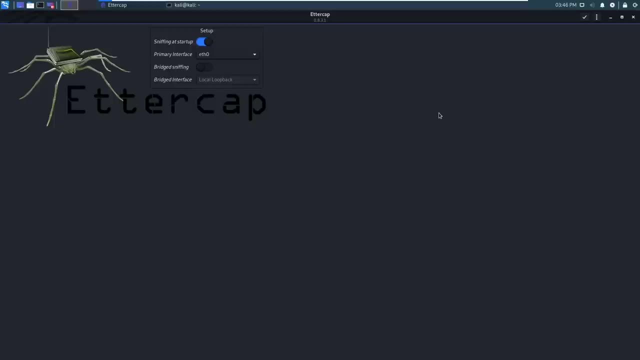 down to sniffing and spoofing. then select Ettercap, I just need to enter the root password and then click authenticate And I'll open this full screen. Okay, so this is Ettercap and this is the program we're going to use to. 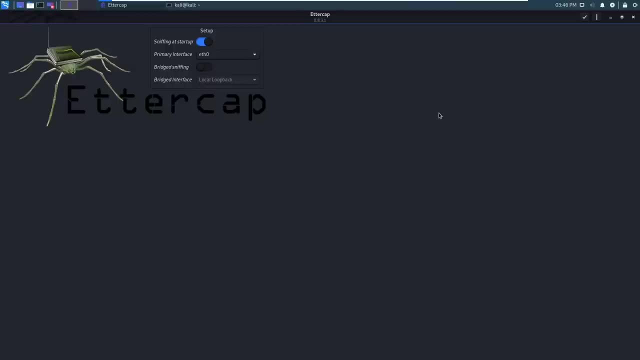 carry out our attack. The first thing we need to do is select our primary interface. EF0 is correct, so I'll leave it selected. Hit the tick button and Ettercap will start up. So now we need to find our targets. The way we do this is by going to the three. 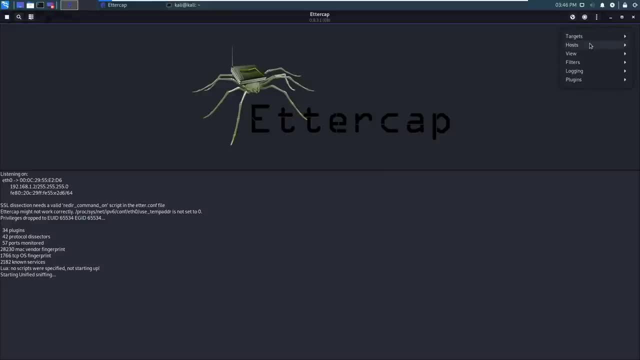 dots at the top of the screen, select hosts and scan for hosts. Now it's going to scan for active hosts. in my network We can see it found two active hosts. To list the hosts, we just need to go back to the three dots hosts and then host. 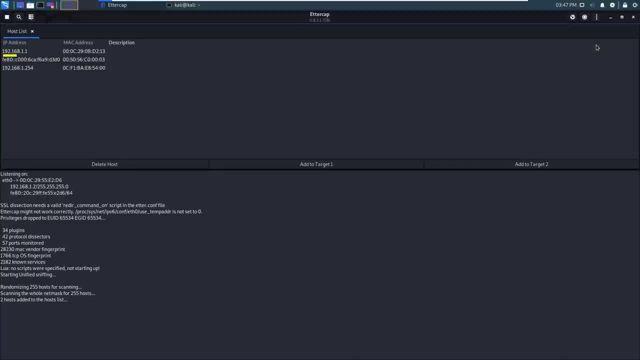 list We can see it has found 192.168.1.1, which will be our victim, and 192.168.1.254, which is our array. I'll first select our victim computer and add it to target one, But for this 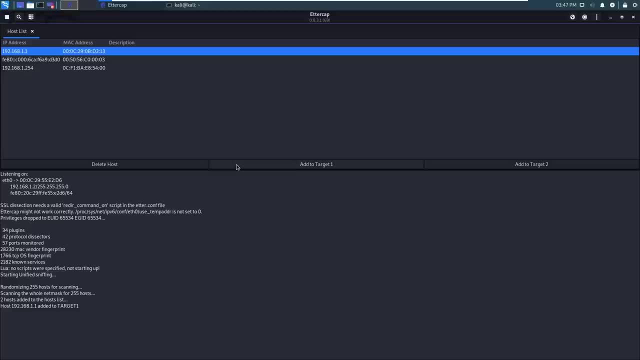 attack to work, we also need to trick the router into sending the traffic back to us and not to the real sender. So we select our router and add it to target two. Now we need to select the man in the middle menu that looks like a little globe and choose our attack. There are a 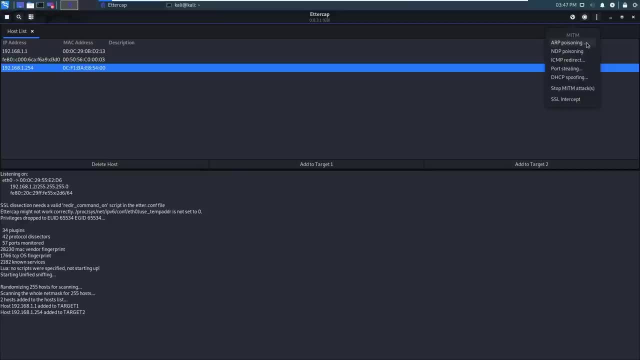 few different options here, but the one we want is ARP poisoning. Once selected, we can select our target. Once selected, you can see at the bottom that it has started the attack. While that's running, I'm just going to open a program called wireshark so we can. 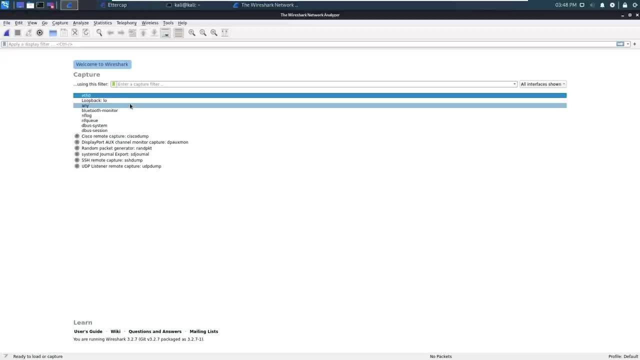 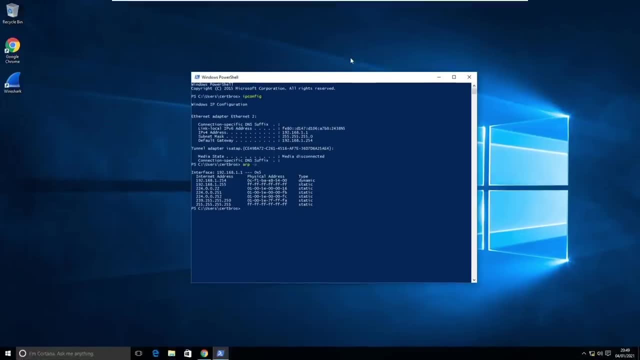 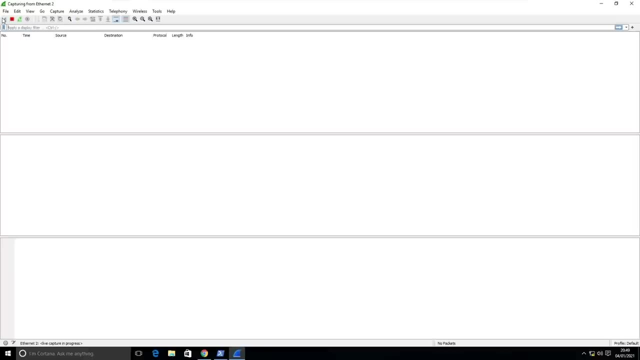 capture some traffic, I'll select the interface and then hit start capture Back to our victim's computer. Nothing out of the ordinary seems to be happening here, but if I open wireshark on this computer, start capture, we should start to see some strange ARP messages. 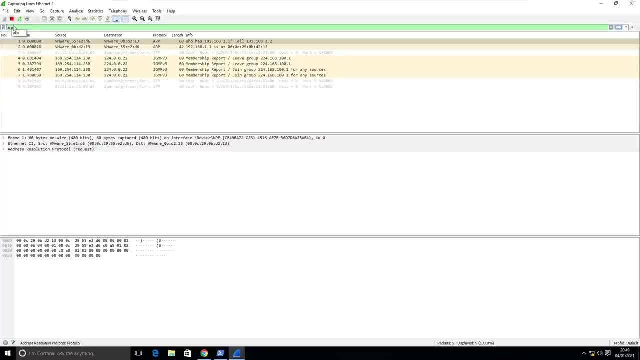 We can make this easier to see by typing ARP in the filter box at the top of the screen. Now, if we wait for a few seconds, we should start to see those ARP messages claiming to be from the router on 192.168.1.254.. But on. 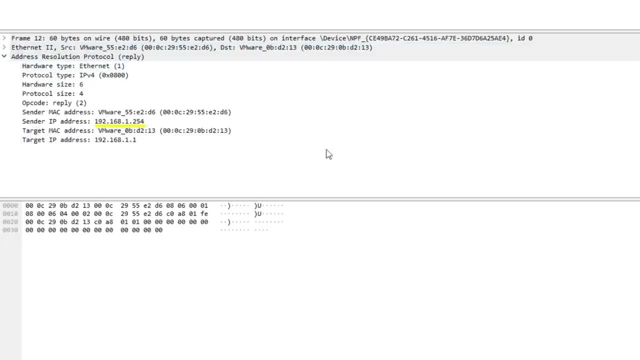 closer inspection we can see the sender's IP address is the router, but the sender's MAC address is in fact the address of our Kali Linux machine. Remember it ends in D6.. This is how it works. This is how it works. This is how we trick our victim, forcing them to update. 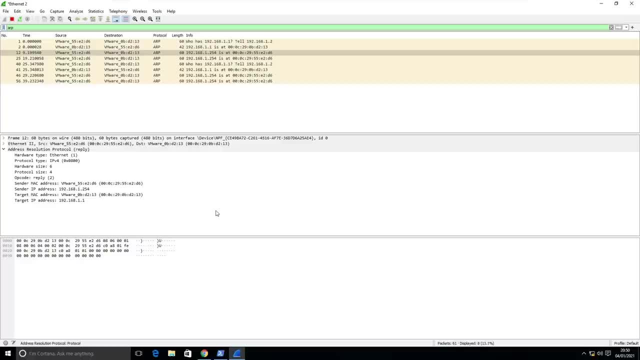 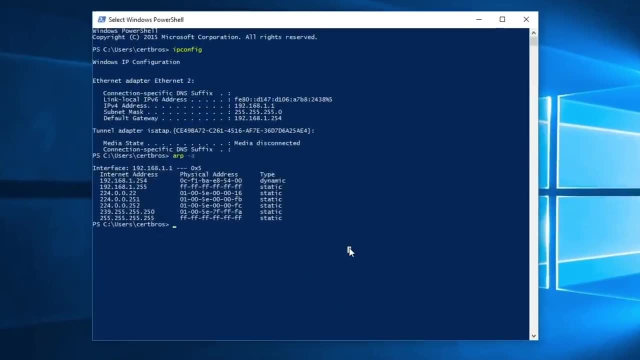 their ARP cache to use our MAC address instead of the real one. To see the effect this is having, let's close Wireshark and go back to PowerShell. If I type ARP, dash A again, we will see the MAC address for the default gateway has. 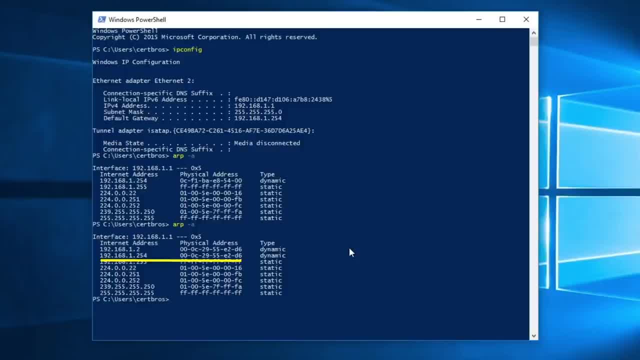 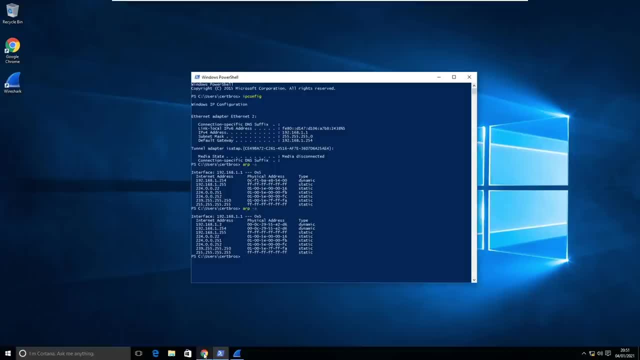 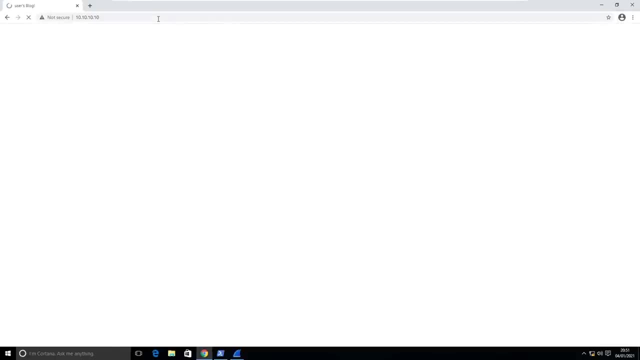 now changed to our attacker's address, Remember D6.. Ok, so now let's pretend we are the unsuspecting user. We open up our web and we browse to a website that is running HTTP and we'll just use this basic WordPress site Because this site is using HTTP. this means all. 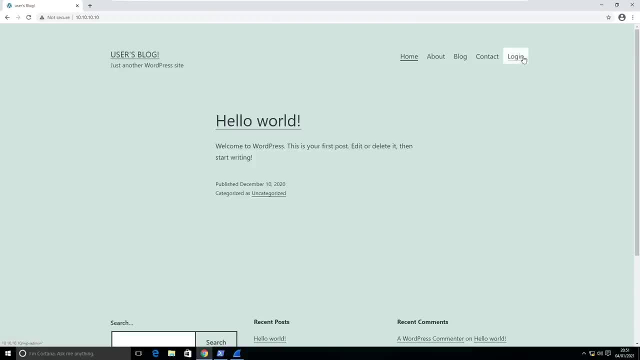 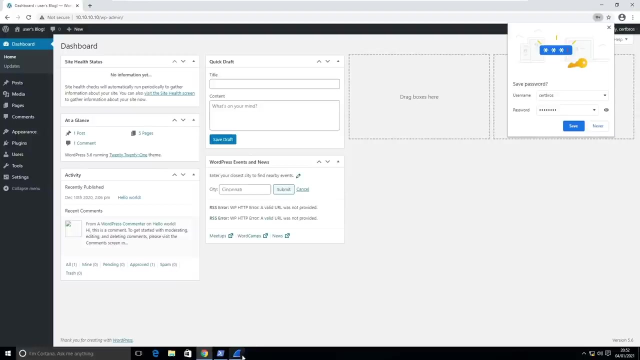 traffic is sent unencrypted. Let's click login, enter our username, then our password, and we're logged in. Nothing unusual happened, right, If we open our Wireshark capture again and this time filter by the website IP address by typing IP address. 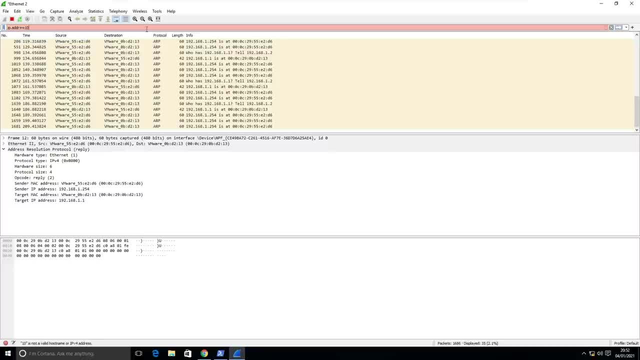 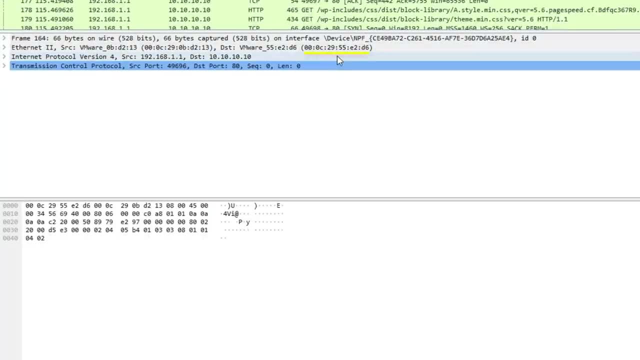 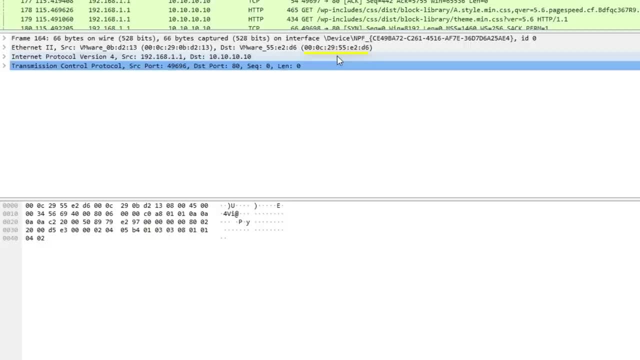 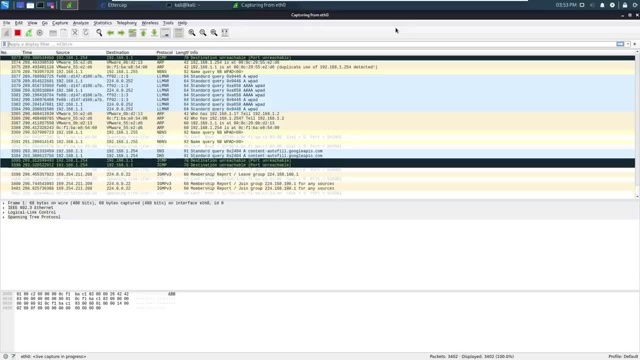 This means all of the website traffic is being passed to the attacker. Let's go back to our attacker's machine one more time. We are still capturing traffic from before. What we can see here is all of the traffic between our victim's machine and the web server. We are 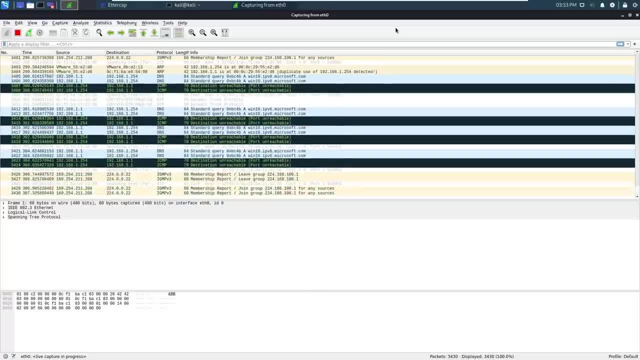 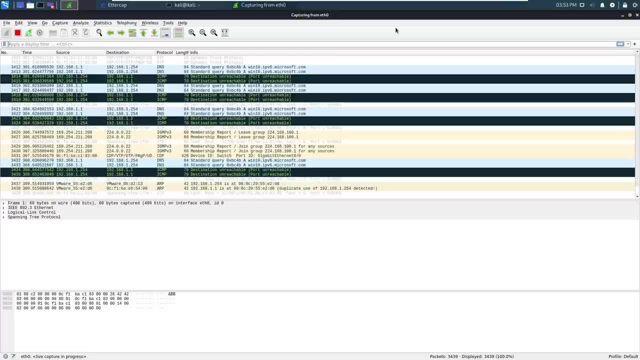 simply intercepting it. This means we can snoop through all of the data that is being sent. For example, I happen to know that WordPress login requests contain the field PWD. So if I use the filter PWD, I can see that the filter PWD is being sent to the attacker. If I use the filter PWD, I 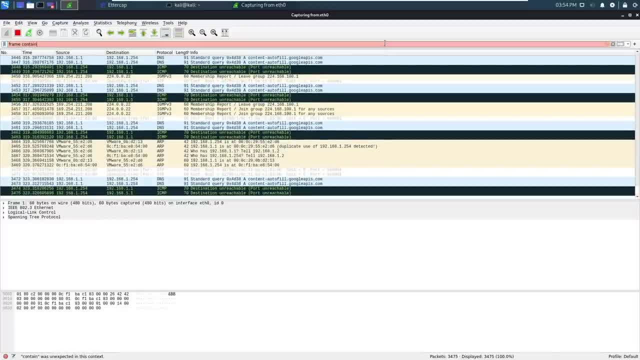 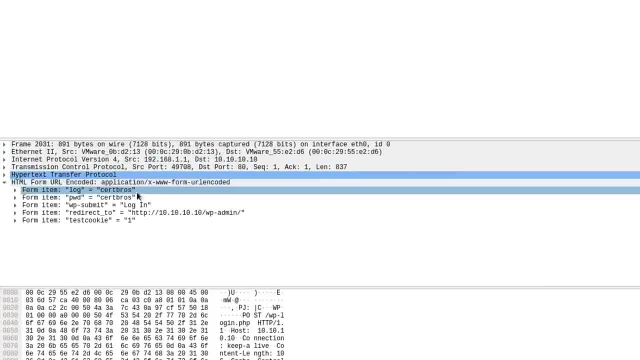 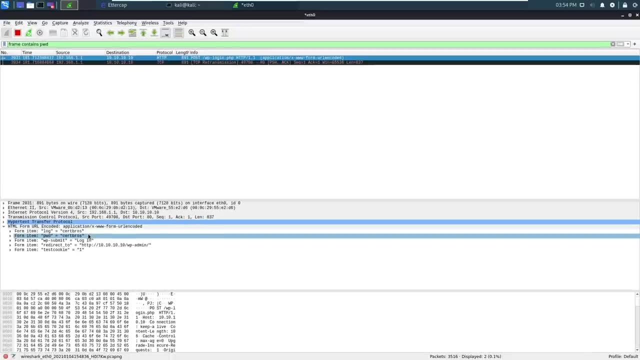 frame contains PWD, we should see the post request. If we then take a look at the HTML data, we can see our login credentials that have been sent in plain text. Now, if you don't fancy searching through huge amounts of packets, then luckily Etikapp does a great job of extracting. 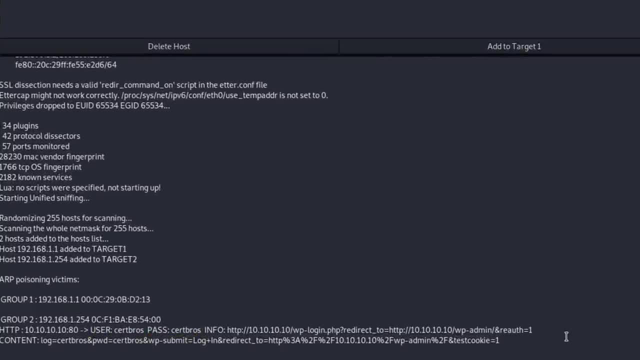 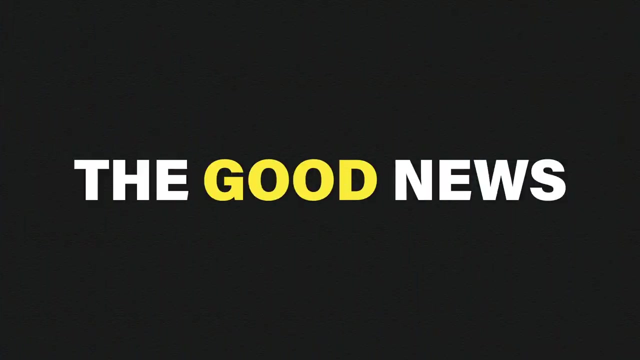 these credentials for us. So that is how we can poison an ARP cache and trick a victim into sending us their data. Then we can extract passwords, files and other confidential information, And that's pretty scary right. The good news is that this type of attack is nowhere near as 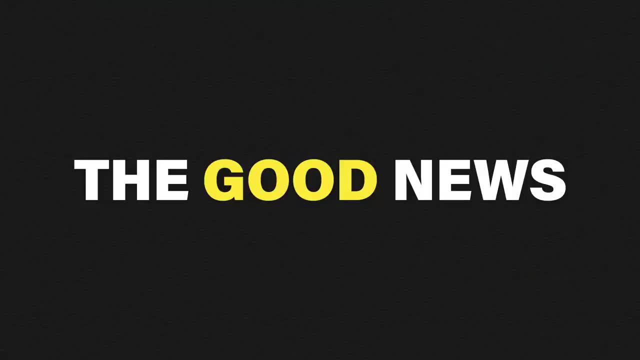 dangerous as it once was. The attack requires the data to be sent in clear text. Protocols such as HTTP, FTP and Tailnet that use plain text have all been replaced with much more secure methods. It's a prime example of why you shouldn't use. insecure protocols. It's safe to say that 90 odd percent of traffic being sent over a network is now encrypted, making this attack largely useless. That said, there are steps we can take to prevent this type of attack from happening in the first place, In particular, dynamic ARP. 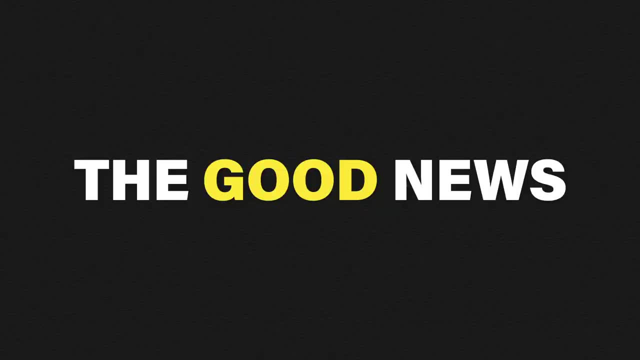 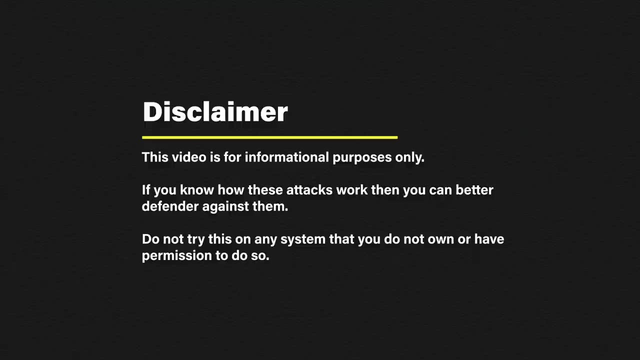 inspection, also known as DAI, is more than capable of stopping this type of attack in a corporate network. Once again, this video is for informational purposes only. The more aware you are, the more secure you can be. Do not try this attack on any systems that you do not own or have permission to do so.